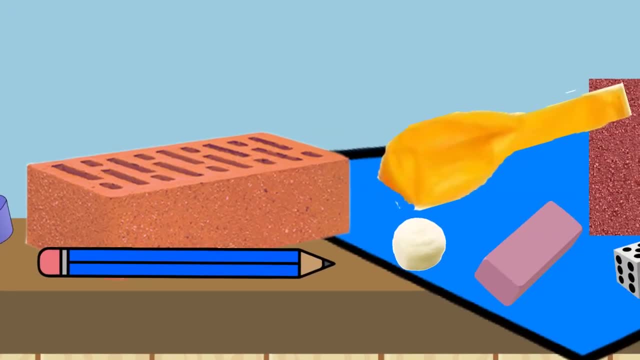 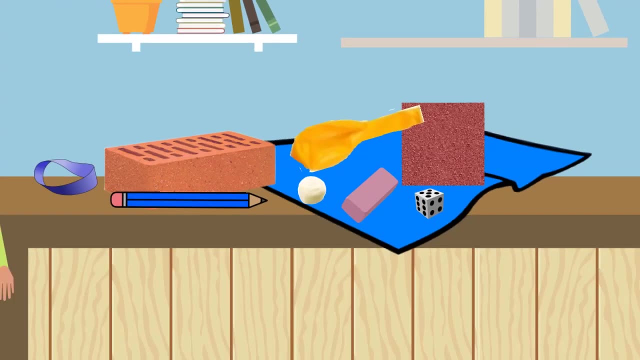 Here we have a rubber band, a brick, a pencil, a cotton ball, a hand towel, a rubber balloon, a piece of sandpaper, an eraser and a single die. Let's start by looking at these objects' colors. Which color do you see the most of? 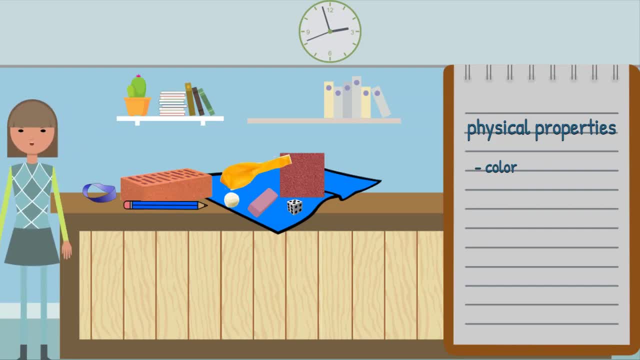 That's right. There are more blue objects than any other color. Color is a physical property we can see or observe. Do you see any other colors? I do too. I see white, yellow, pink and brown. Let's sort out the blue objects. The rubber band, pencil and towel are all blue. Another 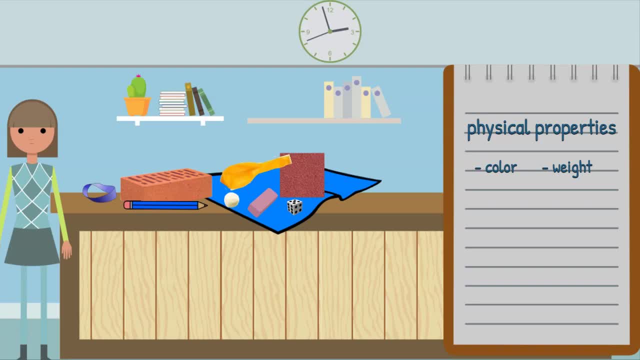 physical property is weight. This can be measured with a scale, but sometimes we can feel differences in weight. Which of these items would be heaviest? Yes, The brick would be heavier than the other items. Texture is another physical property. Texture describes how something feels, Words- 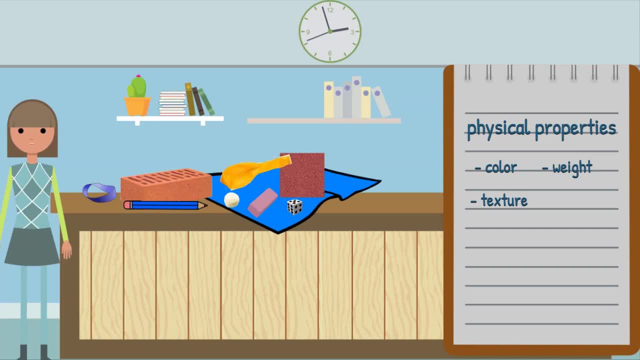 like soft, rough and furry are words that describe texture. Can you name which items are rough? Yes, are both rough. Shape is another physical property. Words like round or square can be used to describe shapes. The brick, sandpaper, die and eraser are all square or rectangle shaped. 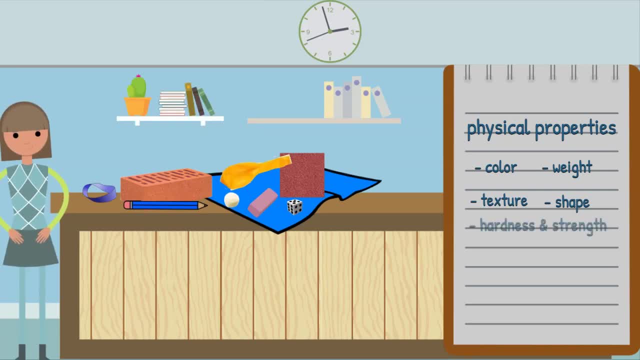 They have straight edges. Hardness and strength are similar but describe different parts of objects. Hardness describes the surface of an object and strength describes the material of the object. They both are used to describe how much force they can handle. A glass has a hard surface, but 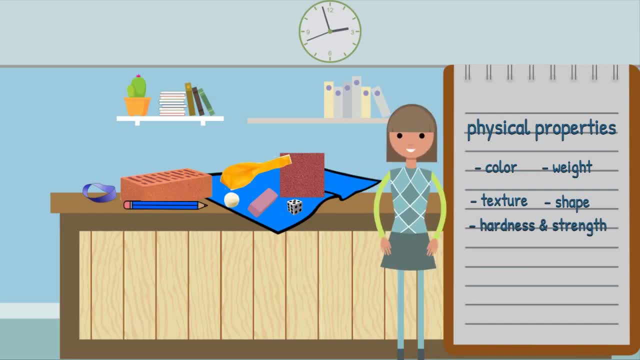 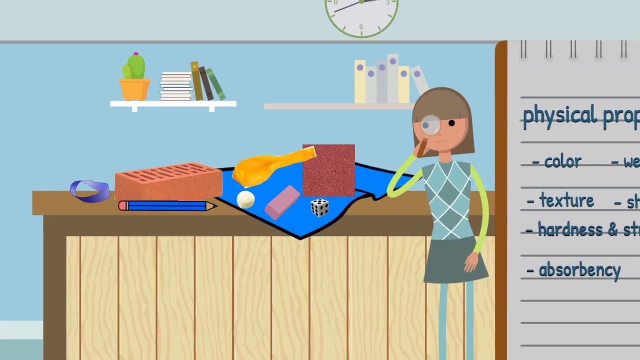 is not strong. If pressure is applied, it will break. Next, let's find objects that are absorbent. When looking at this property, we are looking at how much liquid something can soak up, like a paper towel does with a spill. Which objects would absorb liquid? 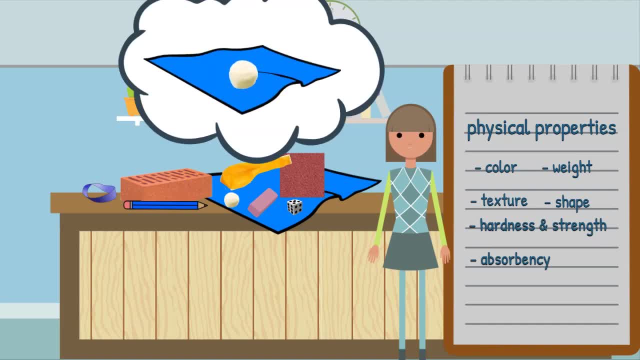 Yes, the towel and cotton ball would both be absorbent. Finally, let's find some objects that are flexible or elastic. These properties describe objects' ability to bend or stretch without breaking. The main difference between these properties is the ability to go back to its original shape.